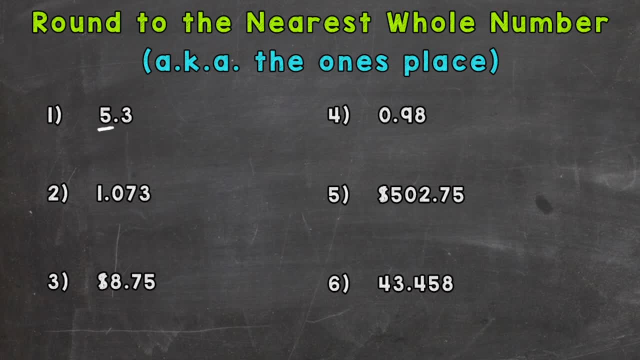 by underlining the digit that's in the ones place, And then we need to look next door to see if we round up or stay the same. Essentially, what's being asked when we round to the nearest whole, is this number Five and three tenths closer to five, or the next nearest whole number which would 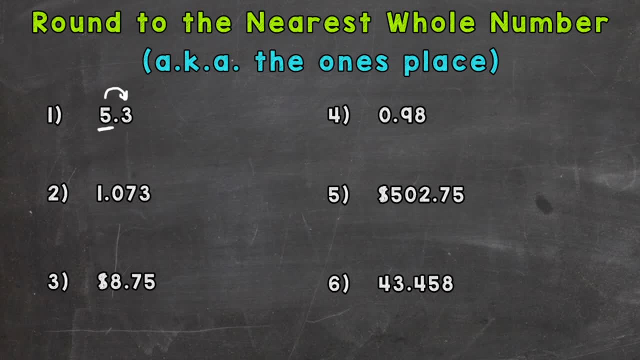 be six. So is that number closer to five or six? So again, we underlined the digit in the ones place. We look next door: Five or more, we raise the score and round up Four or less, we let it rest and the number stays the same. Well, three is less than four. So 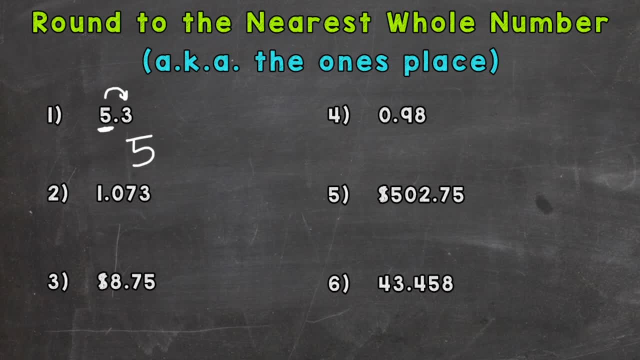 rounding to the nearest whole number. five and three tenths Is closer to five than it is six. So let's take a look at number two Again. nearest whole number is the ones place, So let's underline that. Let's look what digit is next door. 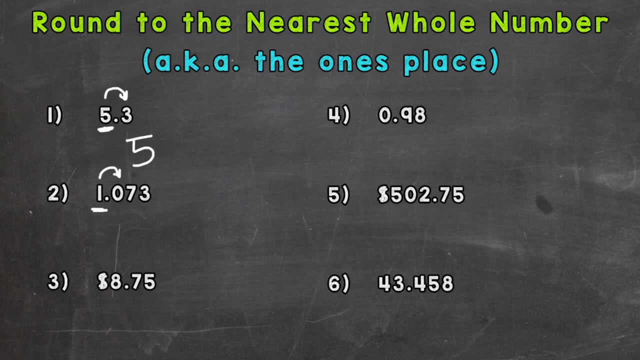 And we have a zero, Five or more, raise the score Four or less, let it rest. So we're asking ourselves: is this number closer to one, or the next whole number, which would be two? Well, that zero says: stay the same. 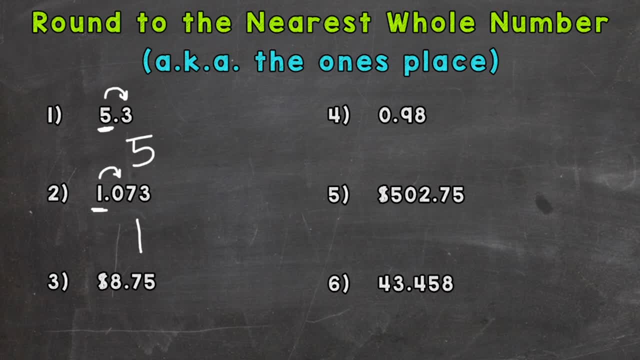 So we're asking ourselves: is this number closer to one or the next whole number, which is the same? So one, Number three: I put a dollar sign there because it's very common to round to the nearest dollar, which is the same as rounding to the nearest whole number or the ones place. So let's round. 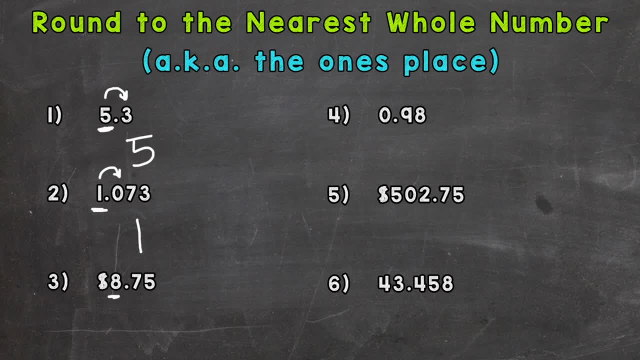 to the nearest dollar or whole number here and underline the ones place. So we're asking ourselves: is eight dollars and seventy-five cents closer to eight dollars or nine? Let's look next door. Five or more, raise the score Four or less. let it rest Well. 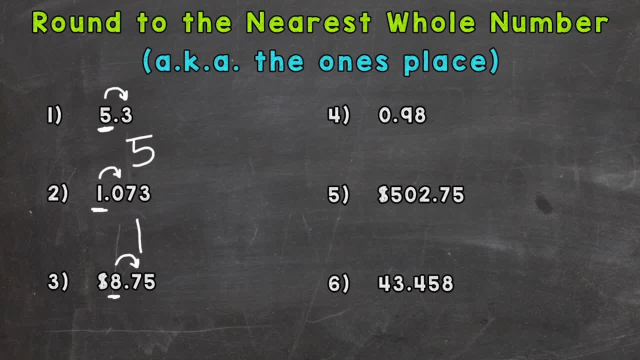 a seven is five or more, so we are going to round up to nine dollars. Number four: we have a zero in the ones place. That's okay. We're asking ourselves: is ninety-eight hundredths closer to zero, or is it closer to one? 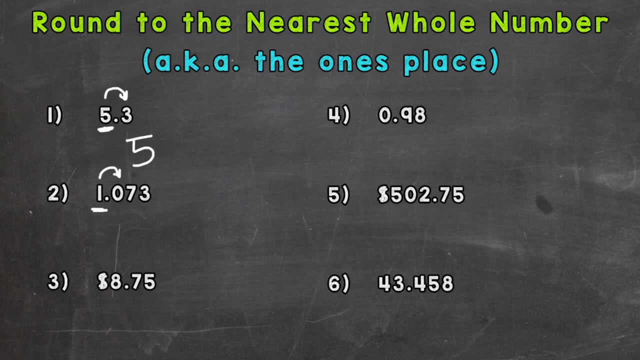 And we have a zero, Five or more, raise the score Four or less, let it rest. So we're asking ourselves: is this number closer to one, or the next whole number, which would be two? Well, that zero says: stay the same. 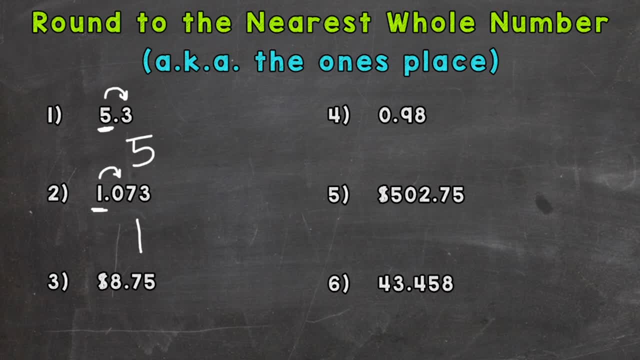 So we're asking ourselves: is this number closer to one or the next whole number, which is the same? So one, Number three: I put a dollar sign there because it's very common to round to the nearest dollar, which is the same as rounding to the nearest whole number or the ones place. So let's round. 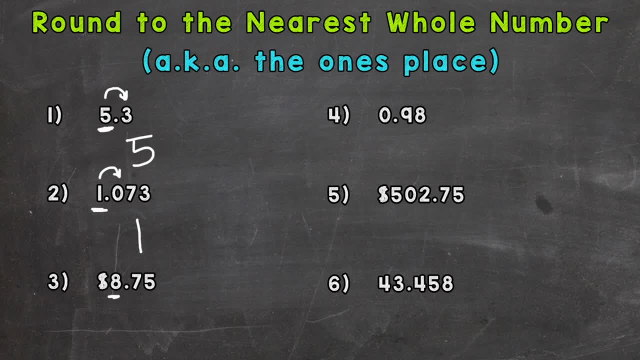 to the nearest dollar or whole number here and underline the ones place. So we're asking ourselves: is eight dollars and seventy-five cents closer to eight dollars or nine? Let's look next door. Five or more, raise the score Four or less. let it rest Well. 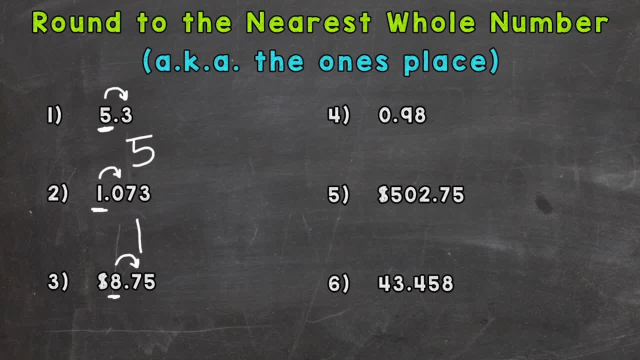 a seven is five or more, so we are going to round up to nine dollars. Number four: we have a zero in the ones place. That's okay. We're asking ourselves: is ninety-eight hundredths closer to zero, or is it closer to one? 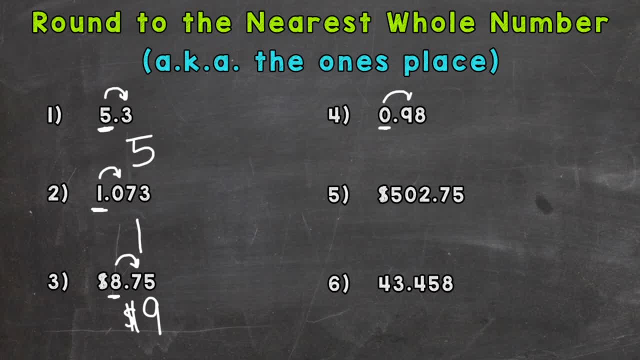 Let's take a look next door and see if we round up or stay the same: Five or more, raise the score Four or less, let it rest. Well, nine is five or more. so we would round up to one Number, five round to the nearest dollar. So we have five hundred two dollars and seventy-five. 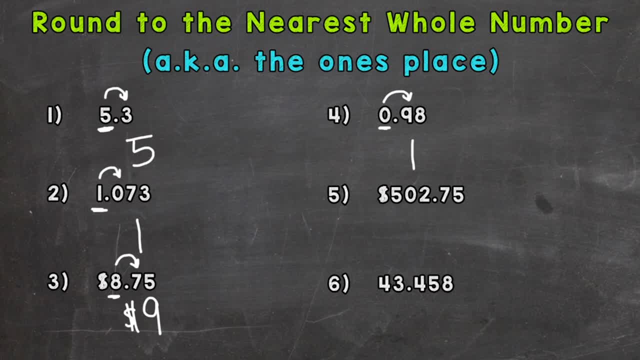 cents. So we need to see if this amount of money is closer to five hundred two dollars or five hundred three. So underline the ones place. Let's take a look next door: Five or more. raise the score there It's a seven. so we round up: This dollar amount is closer to five hundred three. 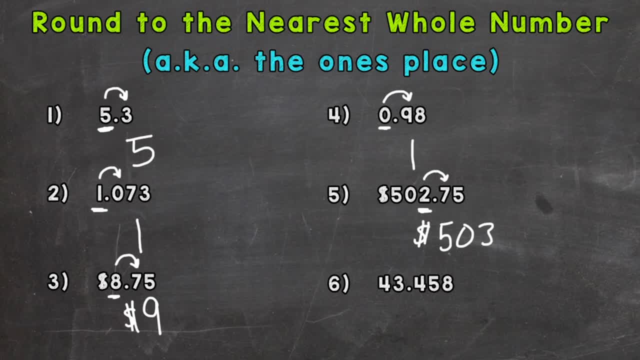 dollars, It would round up to five hundred three. Lastly, number six, we have forty-three and four hundred fifty-eight thousandths. Underline the ones, and we need to see if this number is closer to forty-three Or is it going to round up to forty-four, Four or less, let it rest. So again, we underline.